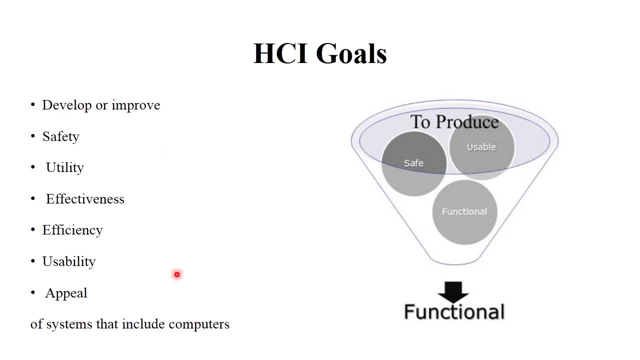 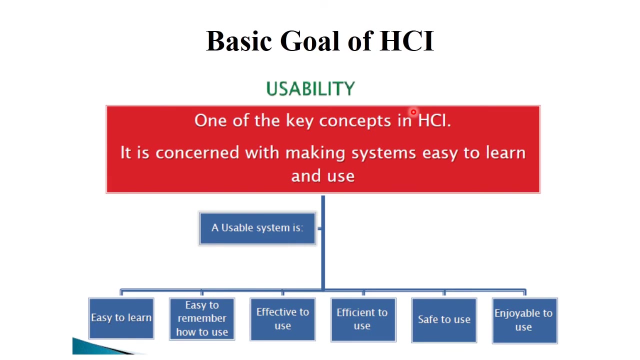 We all are familiar with that. goals of human-computer interaction. Okay, so let's see, one by one, how exactly these goals are work. Okay, next, The basic goal of human-computer interaction Is usability. Usability is one of the key concept in human-computer interaction. 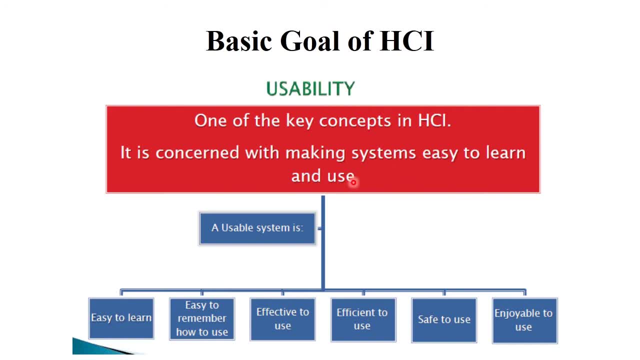 It is concerned with making system easy to learn and use. Okay, nowadays or in real life, the laptops, mobiles, computers, this all things are used in each and every generations, Right from the student to senior citizens, each and every one used all the technological things. 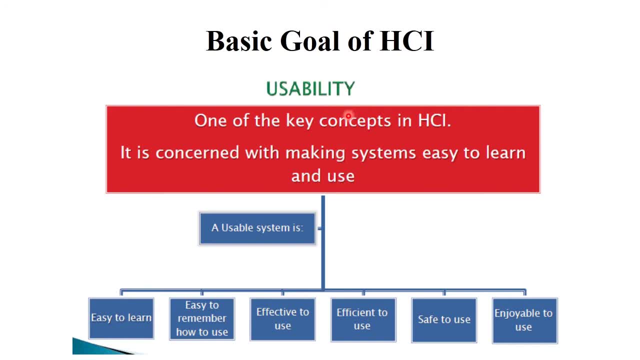 Right, Okay. So usability means a usable system is very easy to learn, easy to remember how to use, effective to use. Okay, when you buy a particular computer, laptop or mobile, you doesn't need any guidelines that how to use that particular product. 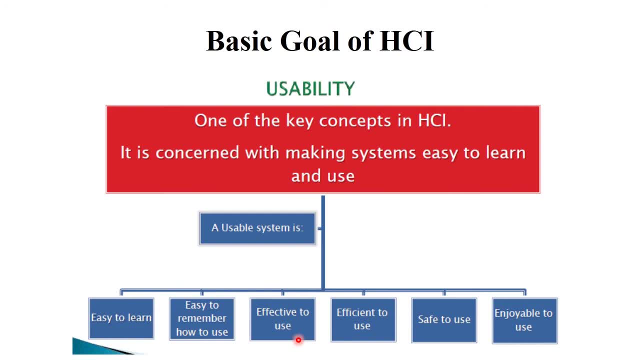 Okay, because each and every operations or each and every button, the particular labels are given. Okay, and from that labels or from that instruction, You will use that particular product Right. You doesn't need any guidelines or any workshop or any seminars of that. 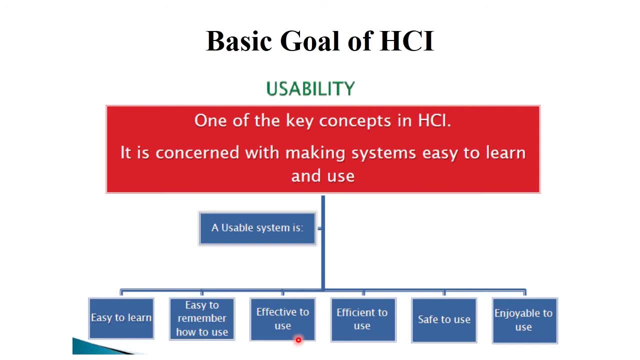 Right Because the system is usable. The computers are usable Right. So meaning of usability is easy to learn, easy to remember how to use, effective to use efficient to use, safe to use and enjoyable to use Right Whenever you are used: the computers, laptops or mobiles. 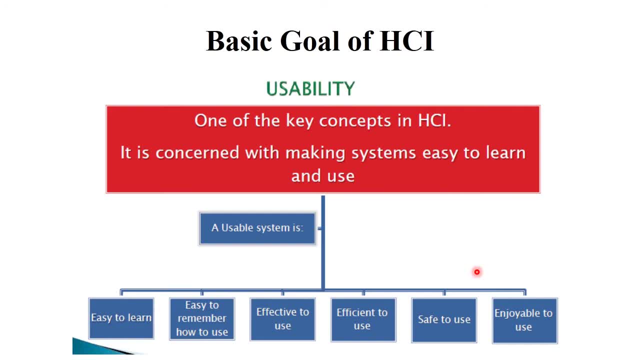 You enjoyed that particular product Okay, And it's very safe for when particular precautions or necessary precautions are taken. It's very safe to use, Right And very efficient and effective for provide the particular output Clear, So which is called as usability. 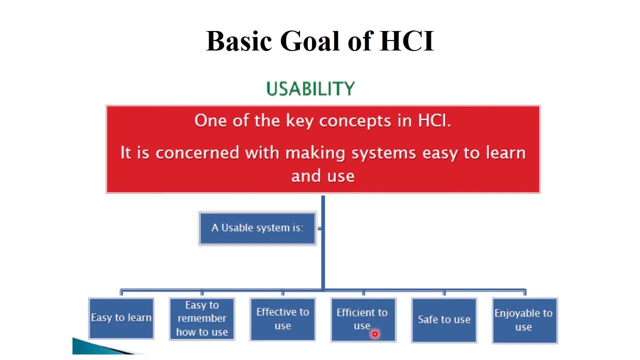 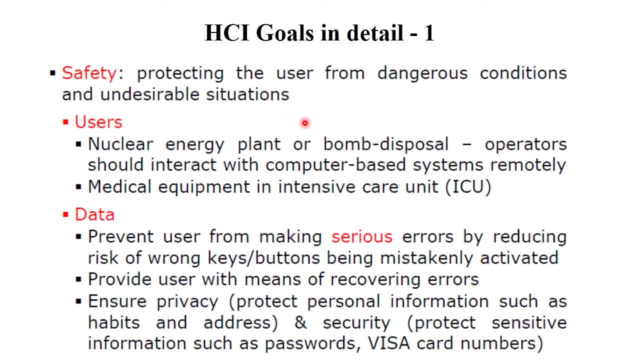 Usability means easy to learn and easy to use, Clear. So this is the basic goal of human computer interaction, that is, usability. Okay, Next, Okay. So next goal of human computer interaction is safety. Nowadays, safety is one of the major issue. 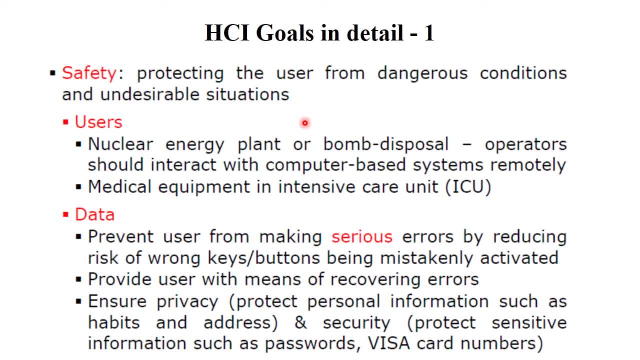 And to handle the safety is one of the most important thing, Right. So safety means to protecting the user from dangerous conditions and undesirable situations. Right, There are also some antivirus apps or other secure things are available. Secure systems or applications are available. 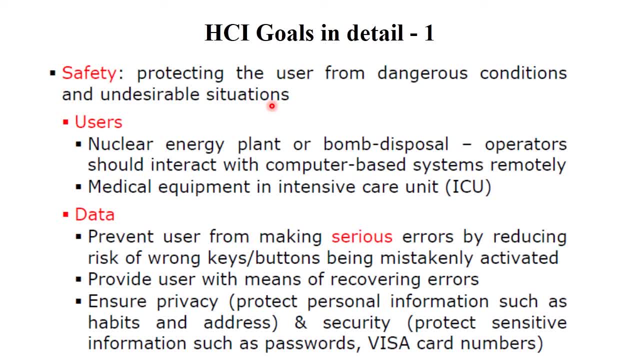 You need to use this, So safety is for necessary. precautions must be taken Right, So which is called as safety. The safety includes two ways, that is, users and data. There are nuclear energy plant or bomb disposal, DRDO, NASA, ISRO. 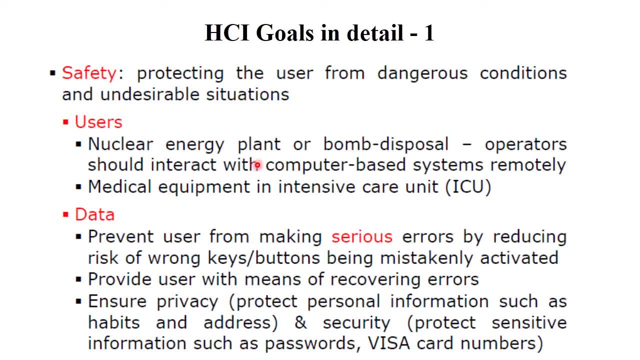 In this kind of organization, safety is one of the major issue Because operator should interact with computer based system remotely Right Medical equipment is also intensive care unit Clear. So through the human computer interaction, safety is provide to the users, to data and 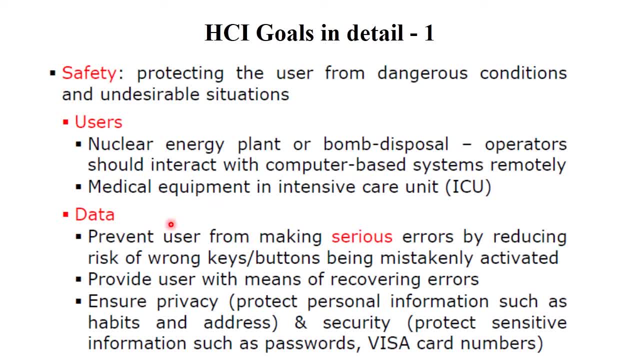 also data to the users, Right. So what do you mean by data? Data means it prevent the users from making serious errors by reducing the risk of wrong key button being mistakenly activated. Okay, It also provide the users with means of recovering errors. 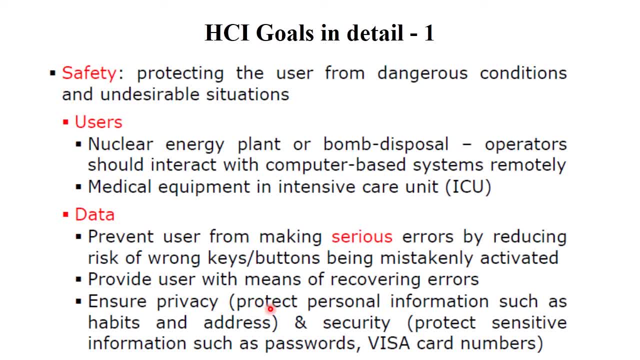 And also it ensure the privacy. Privacy means to protect personal information Such as habits and address, and also security. Security like protect sensitive information such as password, visa card numbers, etc. Okay, So safety must be taken from users to data and data to users. 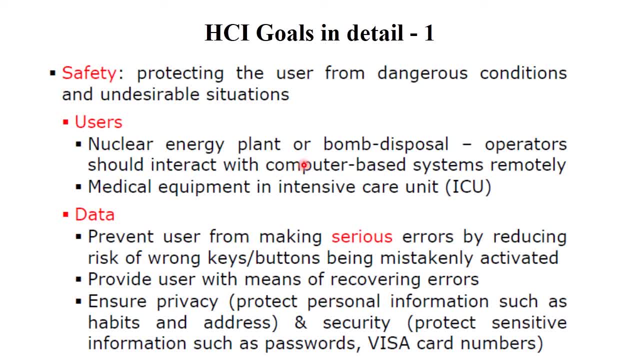 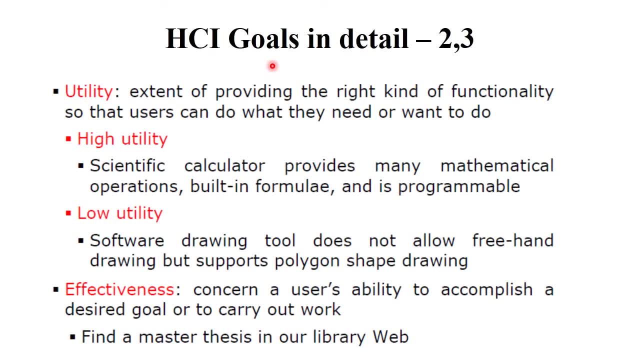 So it's one of the major goal of human computer interaction. Clear, Okay. Next Human computer interaction goal is utility. The utility have two types: High utility and low utility. So for first, what do you mean by utility? Utility means to providing the right kind of functionality. 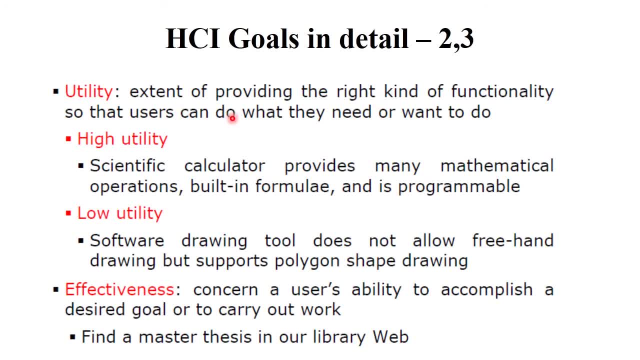 So that users can do what they do or want to do. Okay, Nowadays there are various types of applications are available For browsing: internet browsers, photo editor, video editors. then there are video meetings app like zoom web apps, google meet, etc. 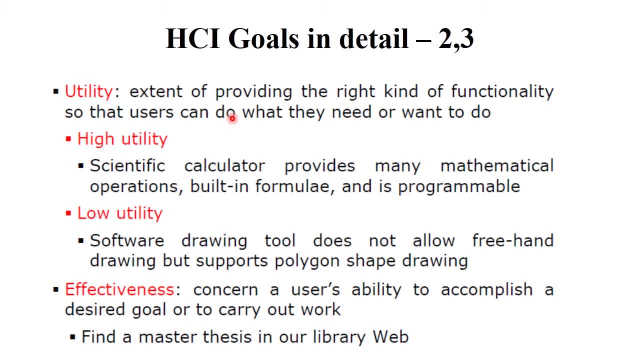 Okay, Each and every purpose, Each and every application, Each and every applications or apps are available. Okay. So utility means to provide the proper functionality to the users as per their requirements. Okay, As per the users requirement: user use that particular app. 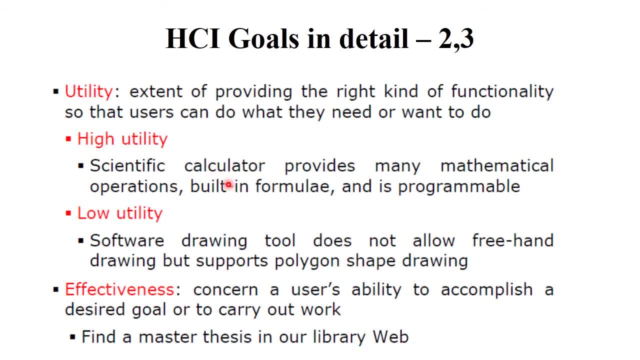 Clear: The high utility means scientific calculator. The one of the example of high utility Scientific calculator provides many mathematical operations built in formulas and it's programmable Right. And low utility means software drawing. It means software drawing tools. There are some software drawing tools. they have there some old libraries and these libraries 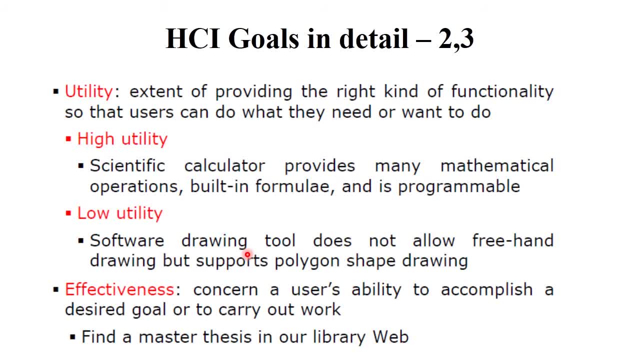 show the different shapes of polygons, circles, square rectangles, etc. But it doesn't provide any or not allow free hand drawing. Okay, So this is called as low utility, Clear The. both high utility and low utility is essential to the user. 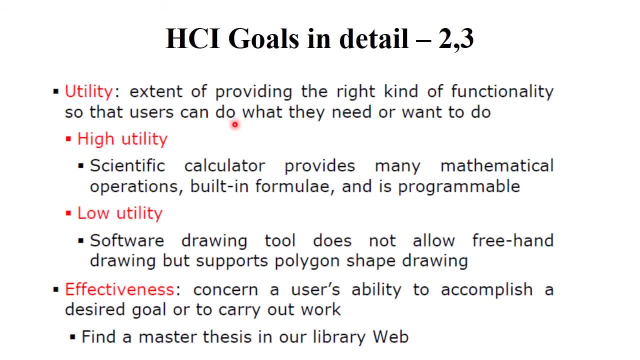 Clear. So utility means to provide the functionality So that user can do what they do or want to do. Clear, Ok. So next goal is effectiveness. Effectiveness means It concerns a user's ability To accomplish a desired goal Or to carry out work. Ok, Whatever, you provide the input to the computers or the mobile. 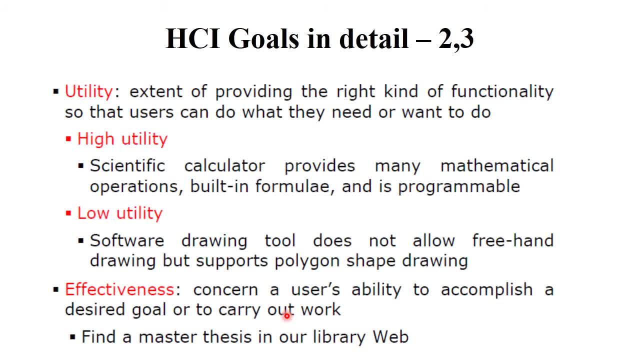 In return, it provides the proper output. Right, If you have to play the music, Ok, Then it provides the particular output That particular songs will be played, Right. So this is called as effectiveness. Proper output will be provided, Clear, Ok. Next. Next goal is efficiency. So what is mean by efficiency? 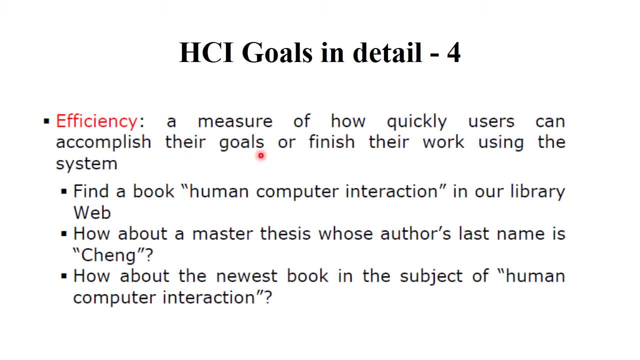 A measure of how quickly users can accomplish their goal Or finish their work using the system We all are familiar with time complexity concept. Ok, For first example is Find a book Human computer interaction in our library web. How to find You just goes on any browser And search on google. 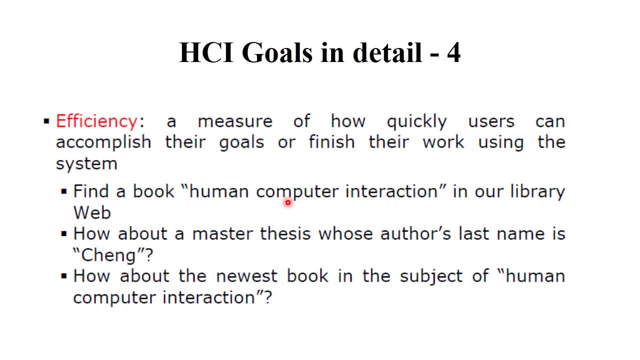 Human computer interaction books, Then it provide multiple links or multiple options, And you have to download this particular book Right, So within a second You have to provide Or you need to perform this particular operation Right So this is called as efficiency. The next: How about a master thesis? 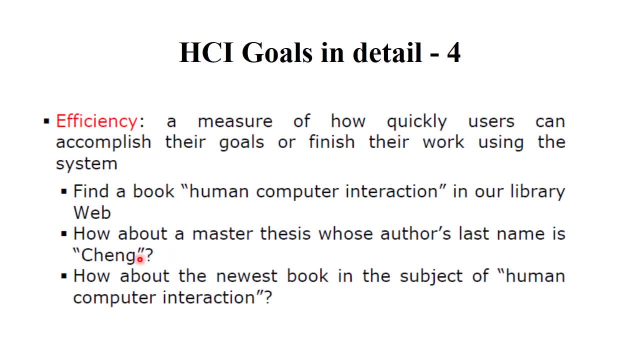 Whose authors love to read and write books, And how about a master thesis whose authors love to read and write books? Their last name is Jai Ok. For that purpose, search operation is used Also. another example is In your contact list in your mobile. You have to search the particular contact within a second. 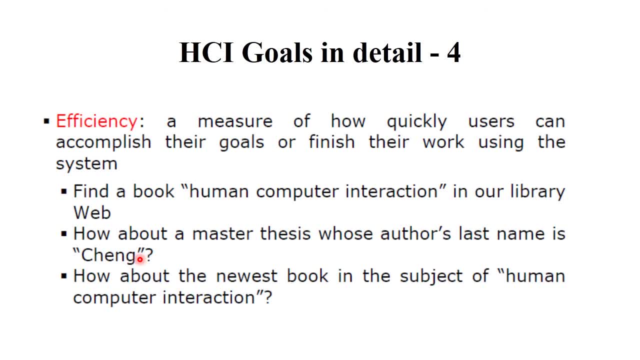 From your contact list, Right, So this is called as efficiency. Means within a second Particular operation is performed- Clear. This is called as efficiency. So efficiency means How quickly users can accomplish their goal Or finish their work using the system Clear. This is called as efficiency. 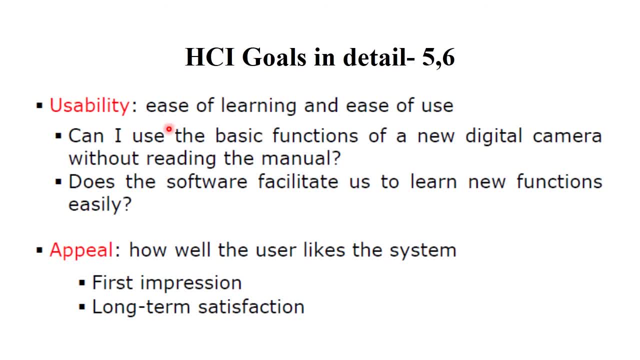 Next goal of human-computer interaction is usability. I already told you about usability. It's one of the key concept of human-computer interaction. So usability means ease of learning and easy to use, Clear Each and every generation, each and every organization or each and every people. 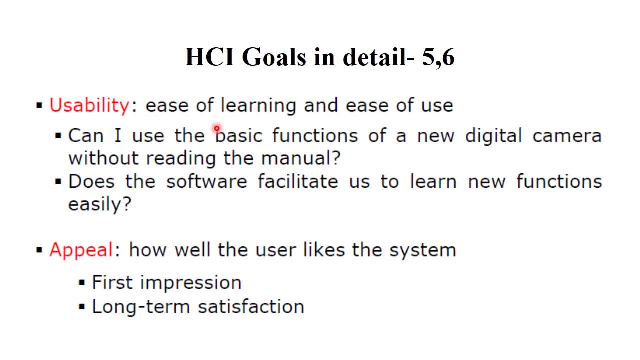 whether the people is technical persons or non-technical persons, for each and every one system is very easy to learn and easy to use- Clear. This is called as usability. The first example is: can I use the basic functions of new digital camera without reading the manual? 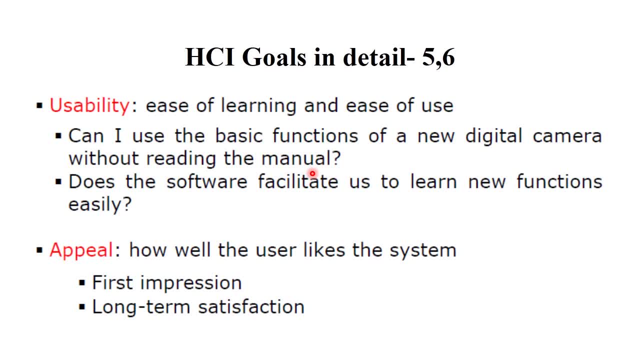 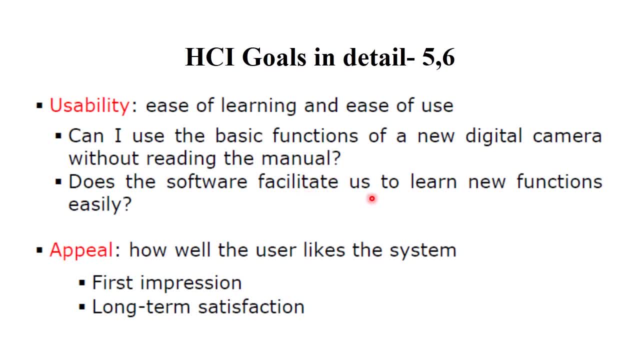 Right, Right, Clear, Clear. Does the software facilitate to use, learn new functions easily? Yes, Each and every software is having some new functions and it's very easy to learn and easy to use Clear. This is called as usability. 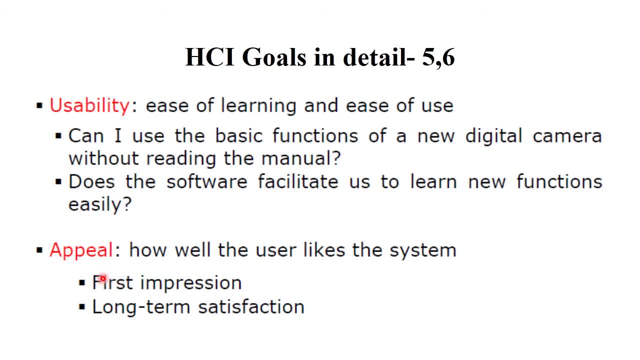 And the last goal of human-computer interaction is appeal. So simply, appeal means how well the user likes the system, The first impression of the users and long-term satisfaction, Right, Okay. Each and every organization, each and every department, computers are used for different operations. Right, In bank, in airline reservation, in hotels, in schools, institute, companies, each and every where systems or computers are used for different purpose, Right. So we just called as appeal. Users get satisfied, Right, And user use that particular thing. This is called as appeal, Okay. 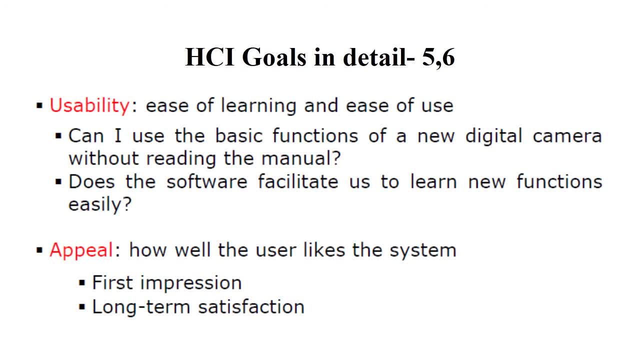 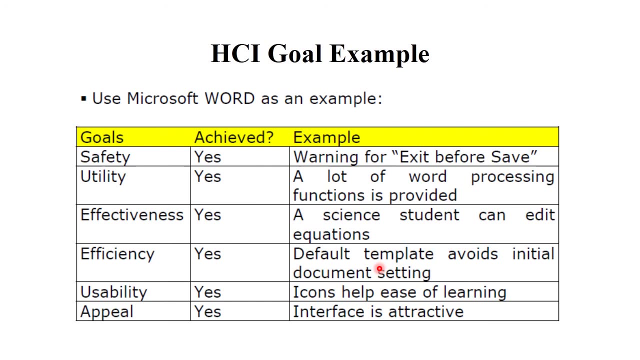 So human-computer interaction, satisfy each and every goal of that towards the user, Clear. So this is all about goals of human-computer interaction. Okay, Next See, here is one example about human-computer interaction goal. Okay, So when you will use Microsoft Word, we all are familiar with Microsoft Word, Right, Let's see. The first goal is safety. 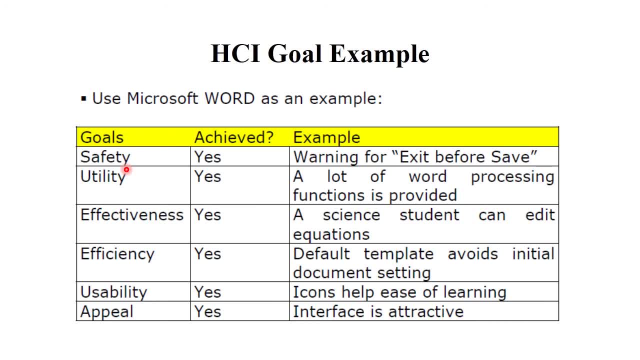 This is interesting: It's Microsoft Word accomplished safety goal. What do you say about that? Yes, Microsoft Word accomplish or fulfill the safety goals. Okay, Because it provides the warning for exit before safe- Right. The next one is utility: These goals also fulfill by Microsoft Word. Okay, Because lot of word processing functions are provided In Microsoft Word. there are different facility or different functionalities- Right. 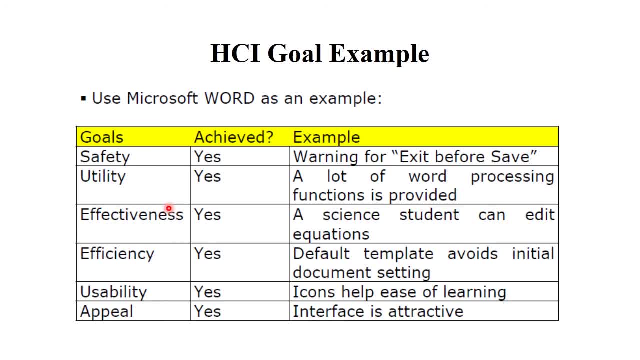 functionalities are available, okay. the next one is effectiveness. yes, this goals also fulfilled by Microsoft Word. for example, a science student can edit equations. right. there are different mathematical equations are provided in Microsoft Word. right, there are different symbols like pi, then summations- these kinds of symbols also provided right, so it's very effective to use by the. 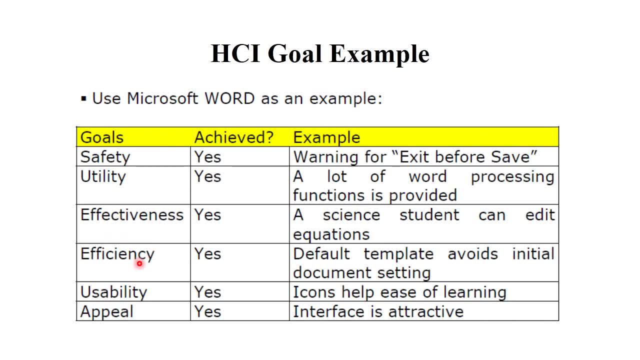 science student clear. the next goal is efficiency. yes, efficiency goal also fulfilled by Microsoft Word because there are default template avoids initial document setting. okay, you need, doesn't need any in, there are initial setting is provided for each and every document, right, you, as per the requirement you. 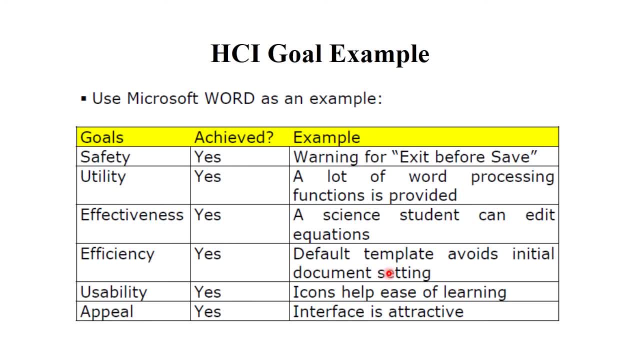 have to provide their margin, their page setup, page border, etc. right. so which is efficiency? the next one is usability. so yes, usability goal also fulfilled by Microsoft Word. because icons help ease of learning, there is cut copy paste of. for that purpose, particular icons are provided right. so by using that icons you perform the particular task right.